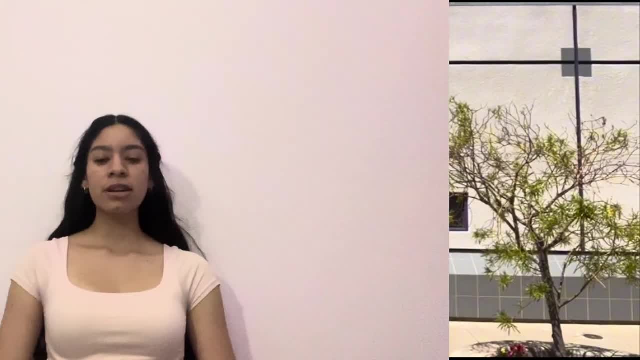 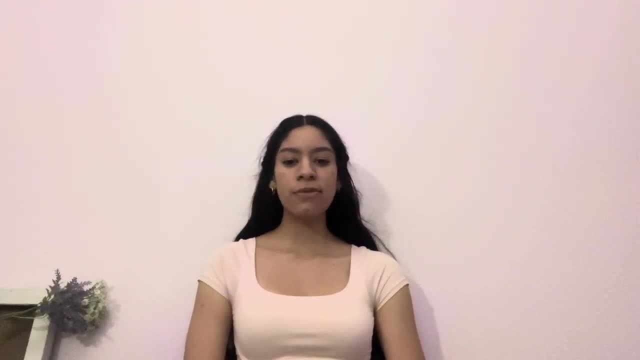 the rocket. the more water the rocket has, the more we'll increase the amount of time the rocket is in the air. The tools that we used were two plastic bottles, play-doh, paint, cardboard and tape. The tools that we used were scissors, paintbrushes and a launch platform. 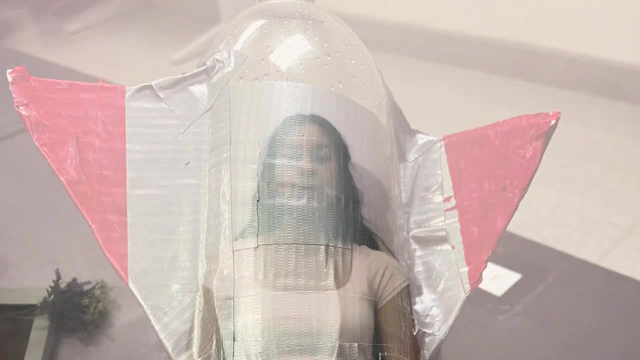 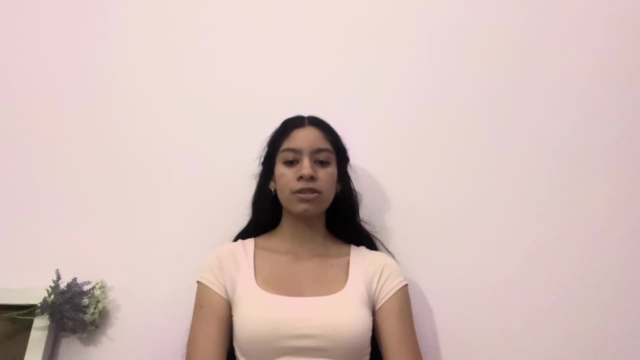 We put weight in the nose cone of the rocket because it's what keeps the rocket balanced. We included fins because it's what provides stability and controls direction. Now, the reason why we put tape around the pressure chamber is to keep the walls from expanding and causing a loss of energy. This way, the rocket will fly at a higher altitude. 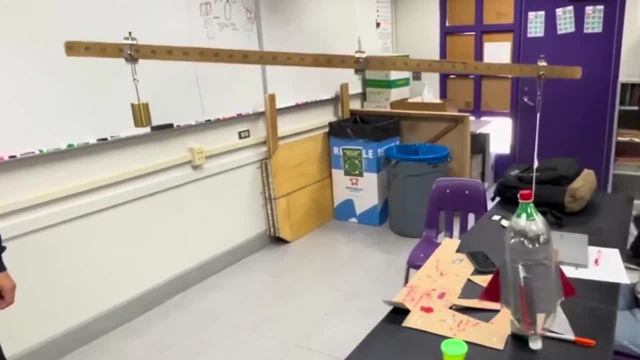 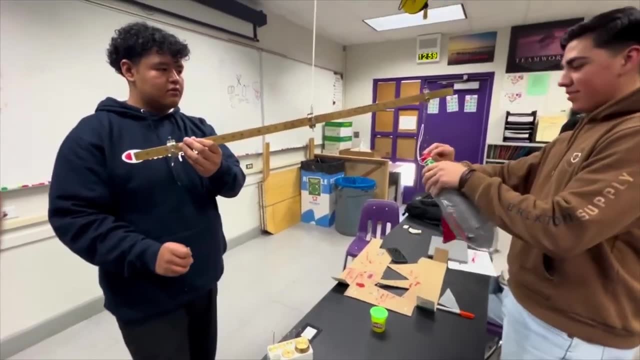 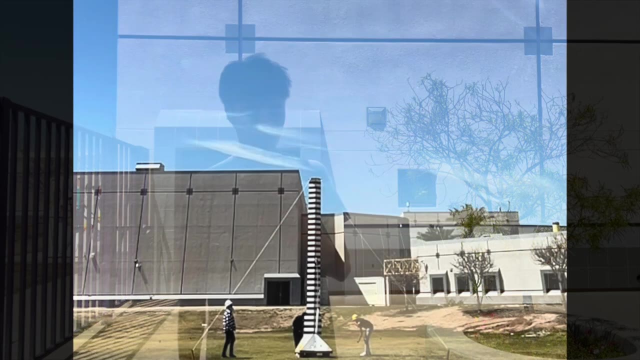 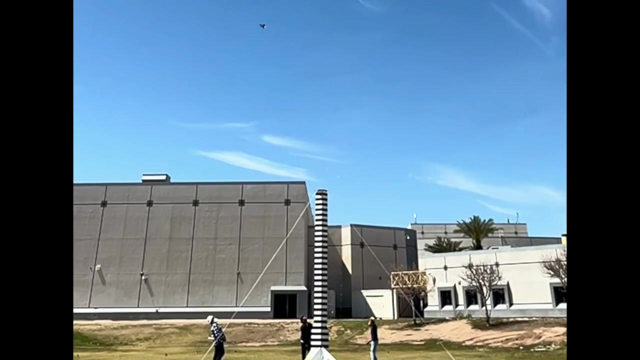 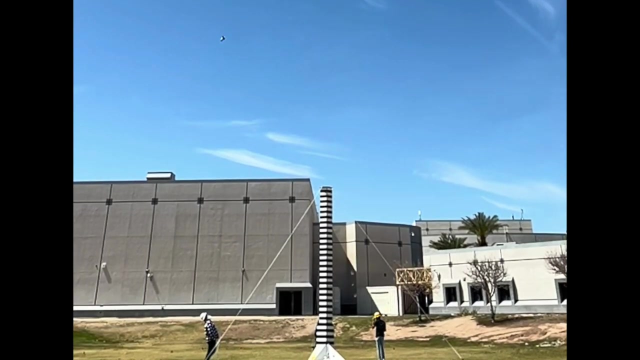 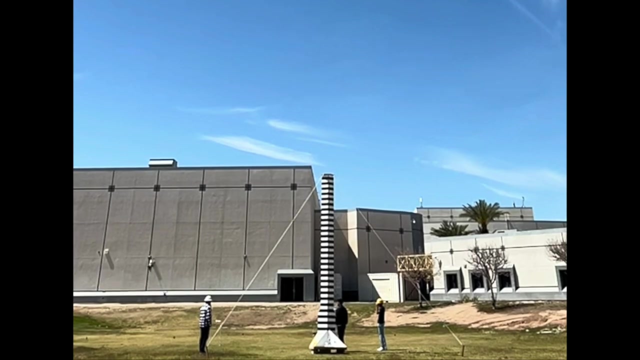 The mass was done by changing the mass on one side until they were both equal. The mass was done by changing the mass on one side until they were both equal. The mass was done by changing the mass on one side until they were both equal. 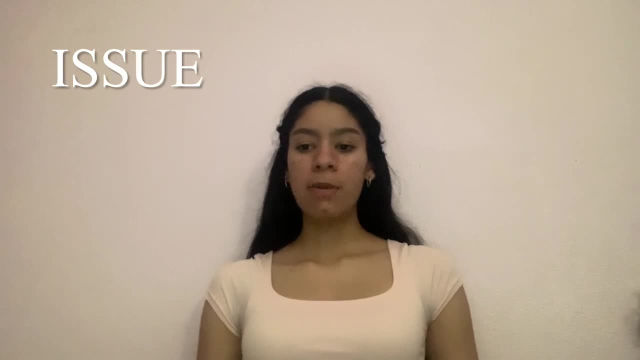 An issue during launch for us was that the rocket hit the rope on its way up, and the reason why this happened was because the fin, or the fins of the rocket, became damaged after every attempt, Since the fins are known to be the guidance system for the rocket. 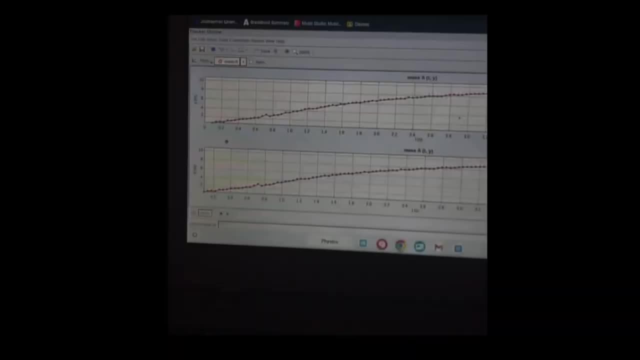 it's highly probable that it would deter from its original straight route. I used tracker online to track the time, to track the distance and to track the speed. I used tracker online to track the time, to track the distance and to track the speed. 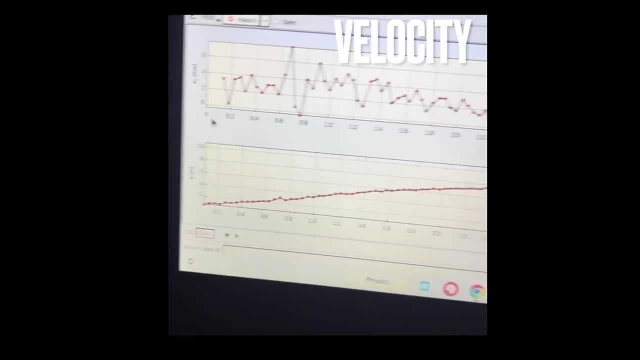 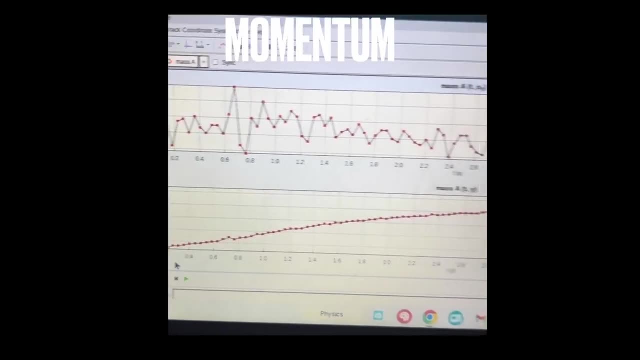 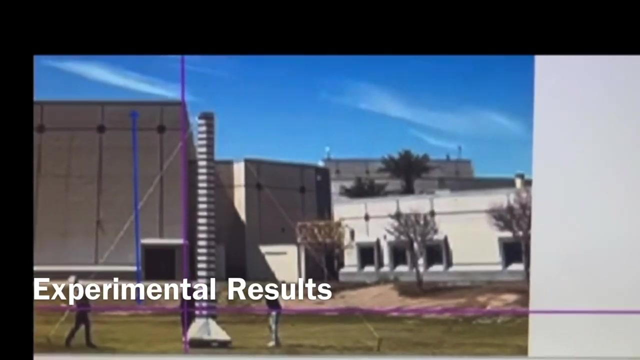 I used tracker online to track the time, to track the distance and to track the speed, To track the velocity, to track acceleration, to track the momentum and to track the kinetic energy And I would say our hypothesis is correct, Although our 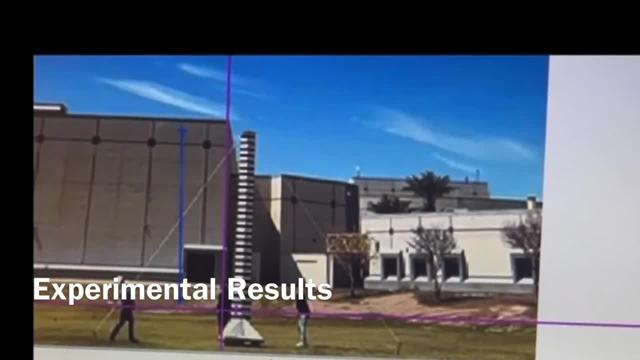 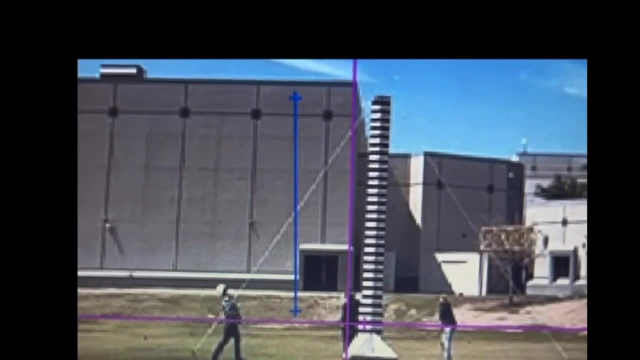 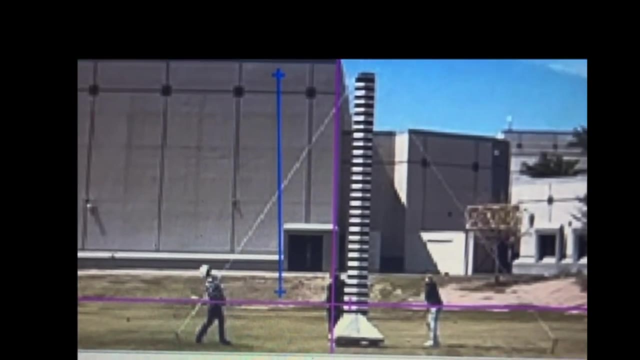 water rocket hit the top of the contraption. it still went pretty high because of the amount of water we put. And the reason the water follows the water rocket is because when the water rocket is launched, the water inside gets expelled out forcefully And, according to Newton's third law of motion, for every action there's an equal. yet 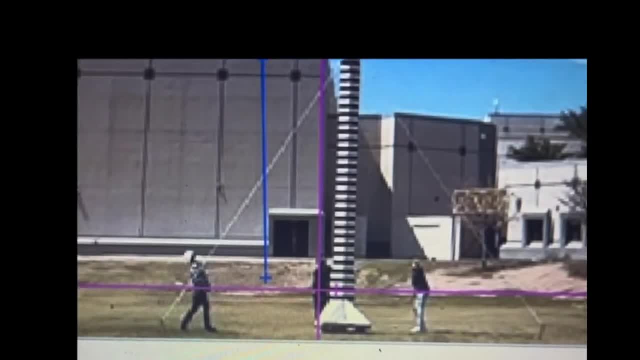 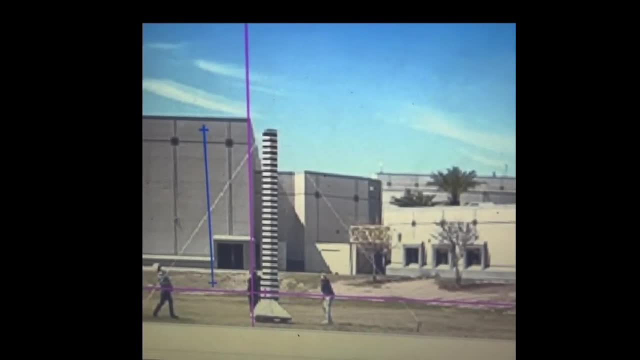 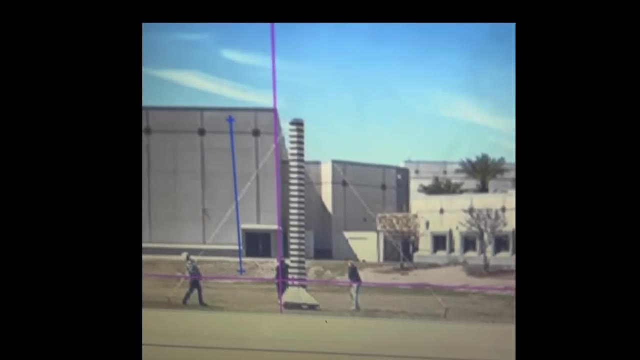 opposite reaction. So when the water is expelled, it creates a backwards force pushing the rocket forward. We learned more about Newton's laws. We also learned about motion pressure and aerodynamics. Something I would say that was difficult would be using tracker online. It was a 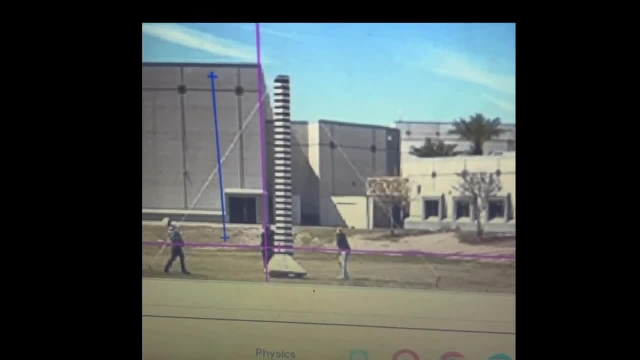 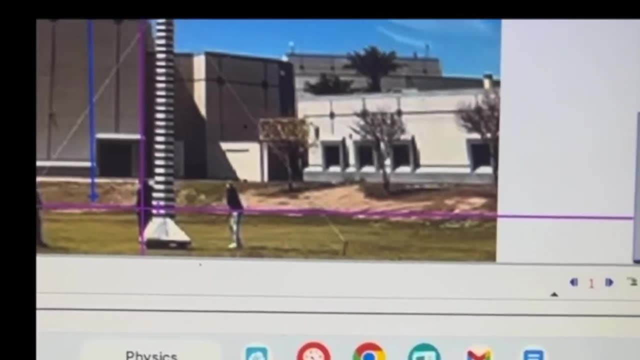 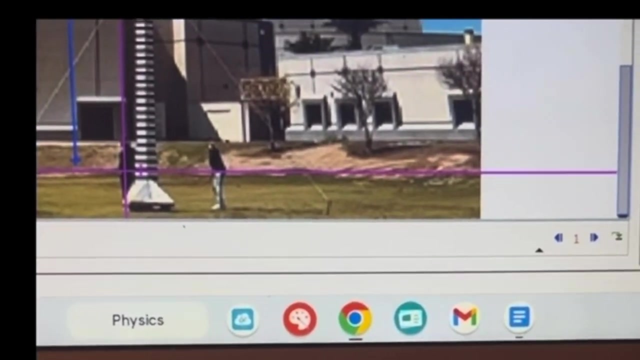 bit confusing at first, but I got used to it towards the end And it was pretty straightforward making our rocket. One thing I would change would be to make our wings straighter and to make them longer. Our wings were pretty short and they were curved, so it would cause our rocket to spin out. 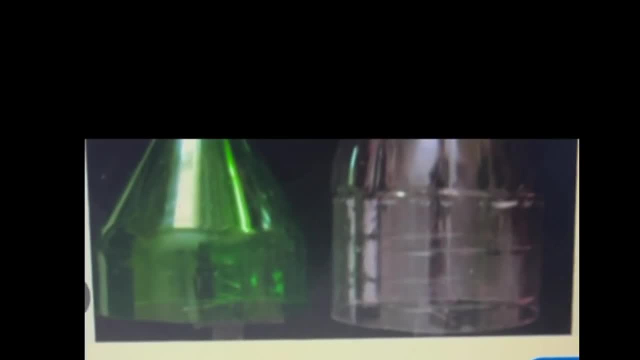 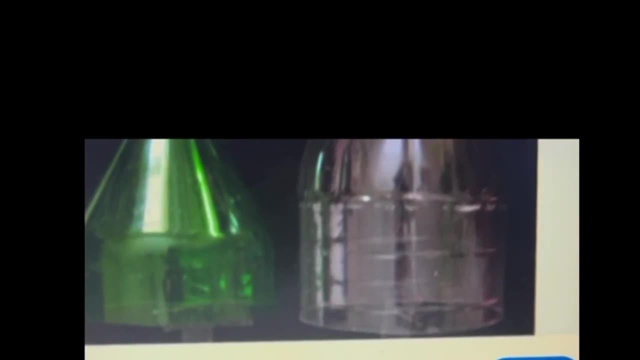 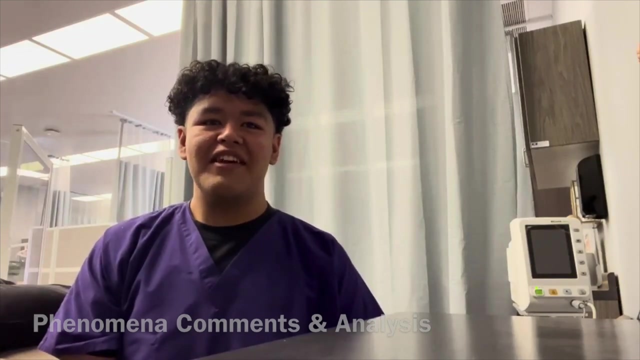 of control. One thing I would recommend to people who are trying to make water rockets is to use a two liter bottle as the rocket's head. We use this size and it is designed intact throughout our experiments, allowing us to conduct more efficient and extensive tests. In the video, as you watch the rocket get launched into the air, you can see. 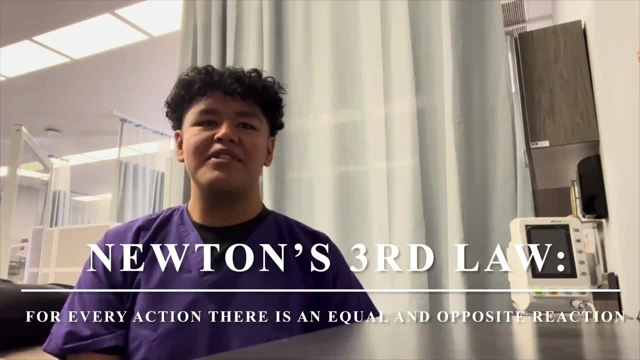 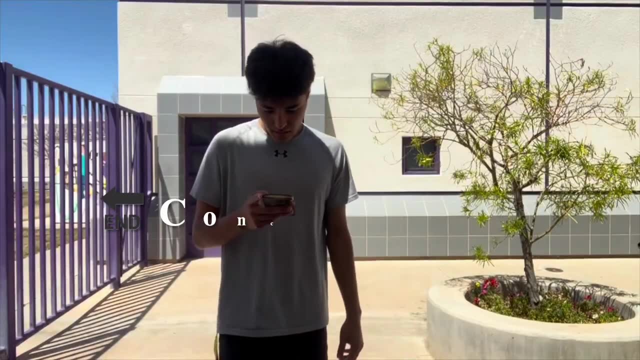 where the water is spewing out from the bottom, It is actually using Newton's third law of motion, where there is a force of air going in and creating an equal and opposite reaction, with the water propelling the rocket upward. In conclusion, something that we learned was that what aerodynamics 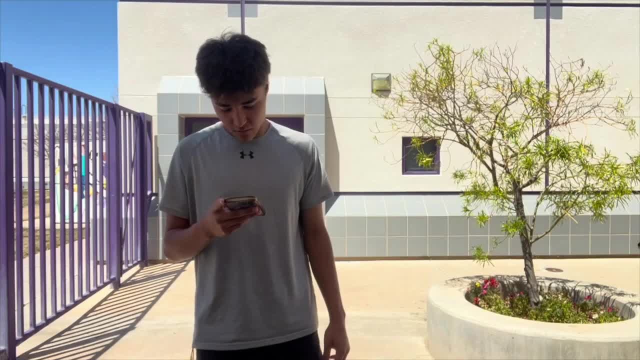 would look like. A difficulty that we encountered was that in the video, the rocket, the rope on its head, would be taking a long and straight line, and then it would get stuck in the air. this way, The rocket would then be able to fly through the air, and their path would be even more difficult. 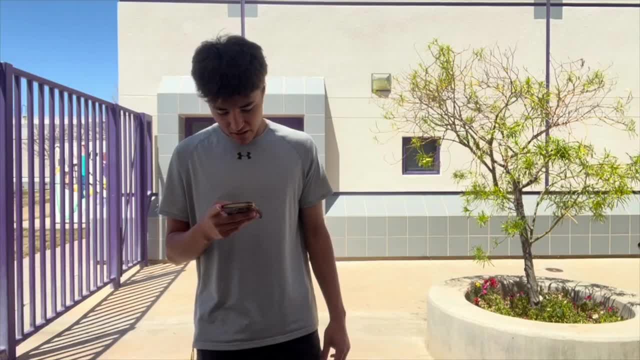 And if we were to do it again and give advice to anyone trying to replicate our bottle rocket, it would be to use more duct tape to make it denser, which would allow the rocket to go further in height. Another thing that we would improve would be the size of our wings, As they were small. 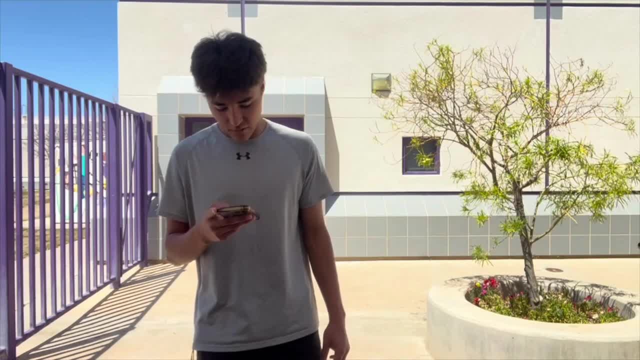 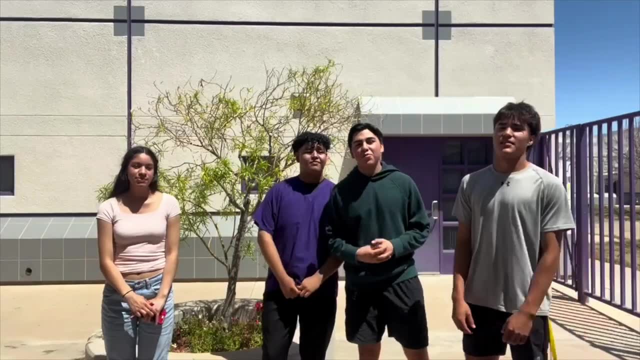 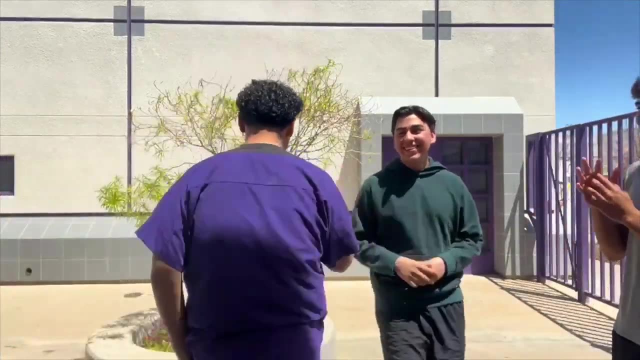